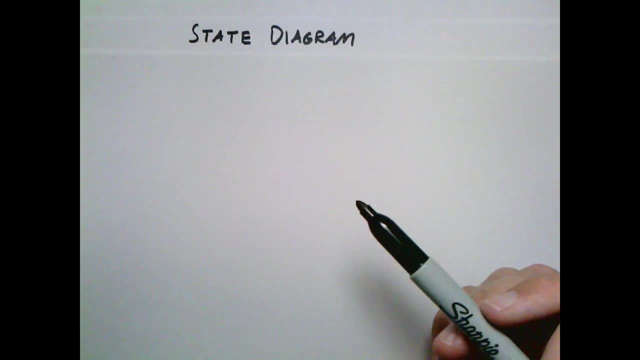 You can use any of these to get your, to get your information across or design your circuit, And theoretically you should be able to, if you know what you're doing, if you understand these concepts. use all four of those things: the logic diagram, the state input equations, the state table and the. 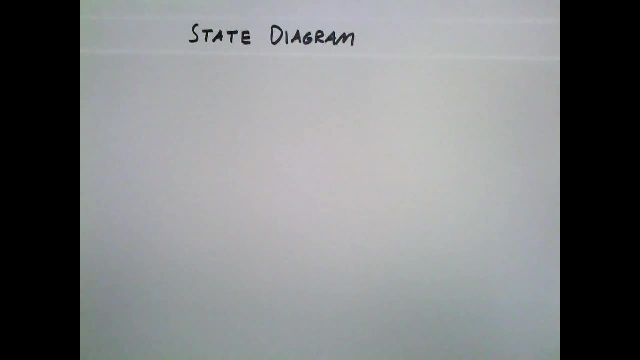 state diagram. Basically, if you have one of those, you should be able to get the other three, because all that information is still there. So, but, like I said, let's jump into the state diagram and talk about that and how that works. And so basically, we just draw. remember we had A and B, our 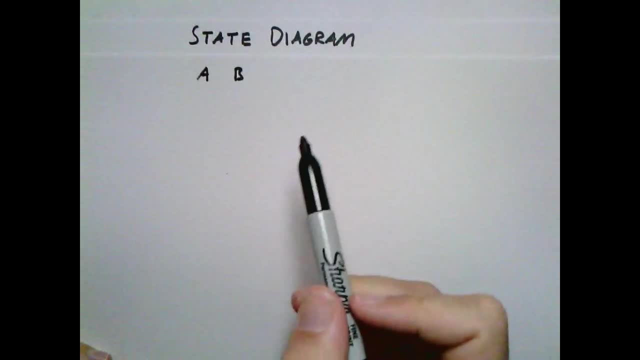 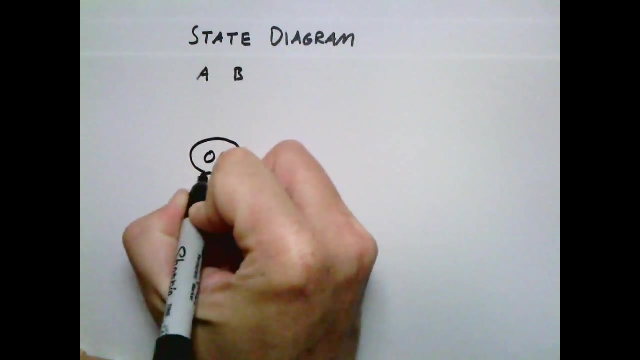 states are A and B, which means our we have a two bit value here, which means we can only have four states. Our system, our circuit that we've been looking at, can only have four states. right, Zero, zero, draw a little circle: zero one. 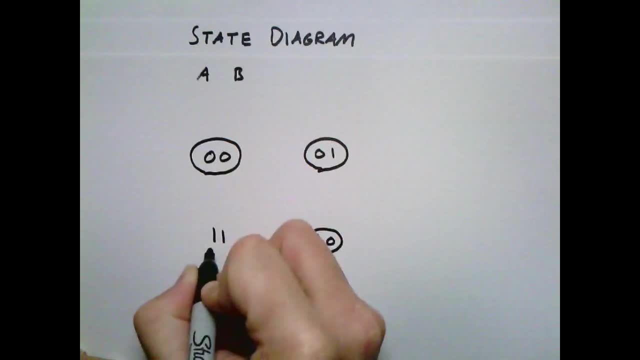 one zero and one one right. Those are the three states that the circuit can take, And so, from there, all we do is we sort of take our diagram and go from there. So let's bring that in real quick. So let's start. 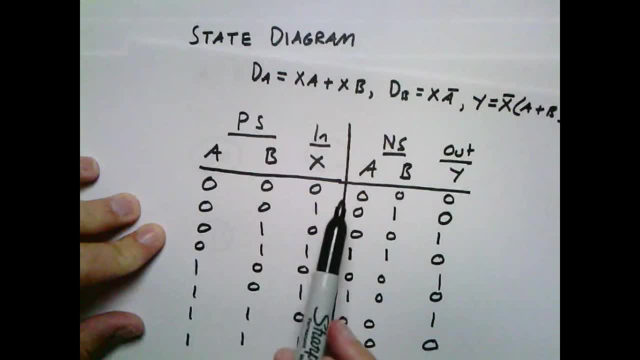 at state 0, 0, which is right here, right 0, 0, 0, 0, x is 0 and x is 1.. And we say: well, when we're in state 0 and our input is: 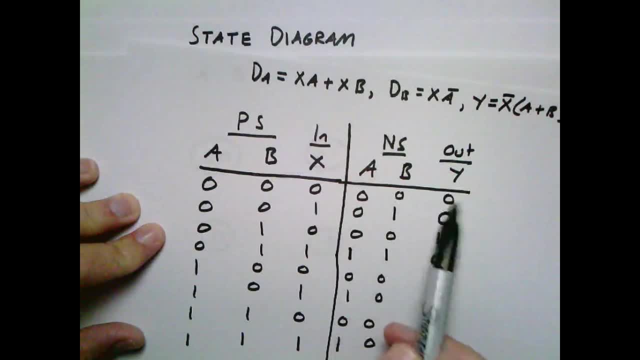 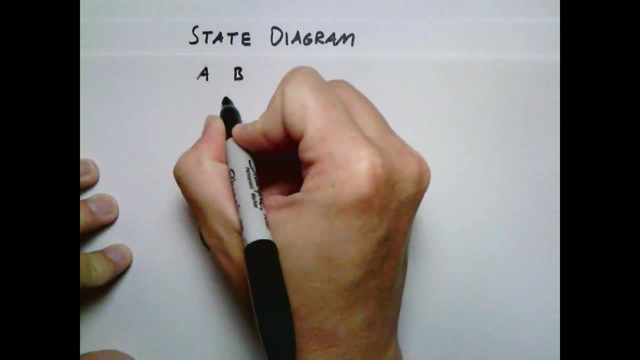 0, then our next state is 0, 0 and our output is 0. So what we do is, since we're going back to the same state, we'll just draw a line that sort of loops back on itself, back to 0, 0. And then there's a little bit of 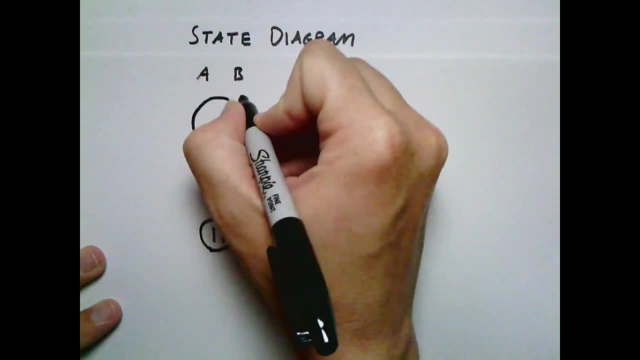 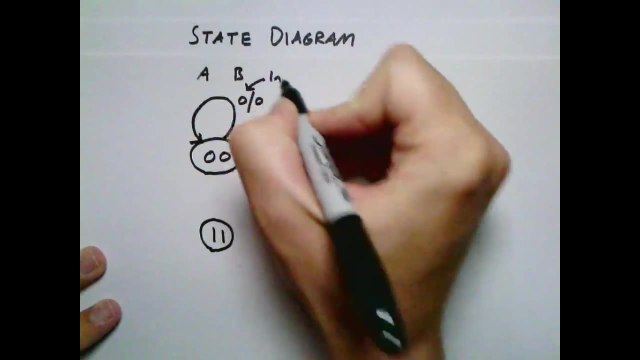 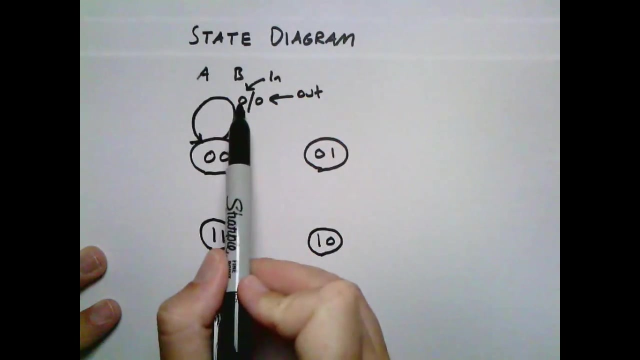 notation here. Basically, we'll have a number, a slash and then another number, And the first number, that's our input. The second number is our output, And so we just know that if we're at 0,- 0 and we get an input 0, we're going to go back to state. 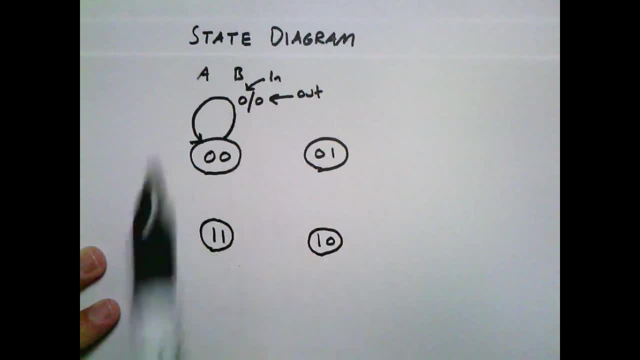 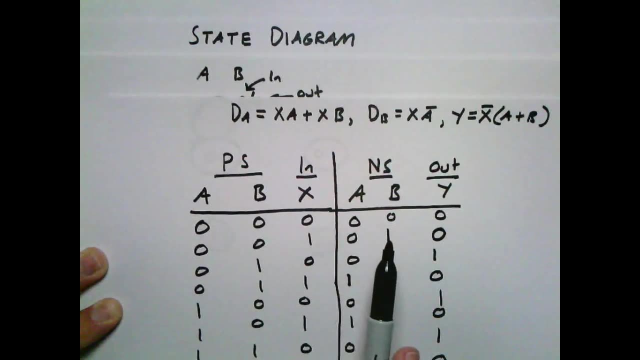 0 or stay at state 0 and we're going to output a 0.. Now, looking at the diagram again, if we're at 0, 0 and we get a 1, we're going to go to state 0, 1 and still output a 0.. 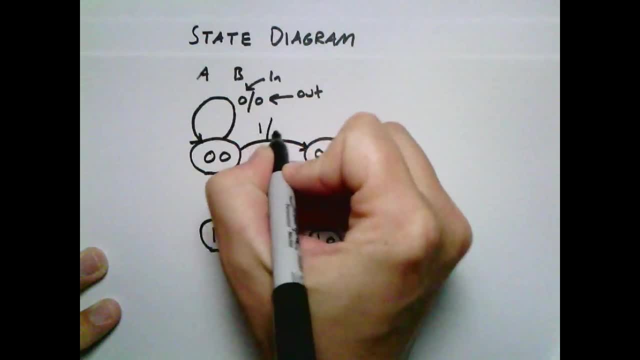 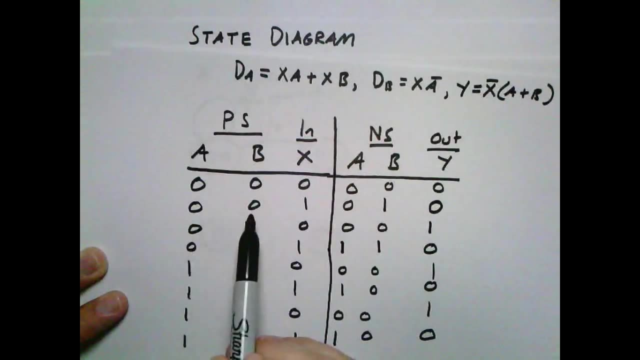 So we're going to go to 0, 1 and we're going to take 1 as input and we're still going to output a 0. And that's it for 0, 0.. Now 0, 1, you can see we have 0,. 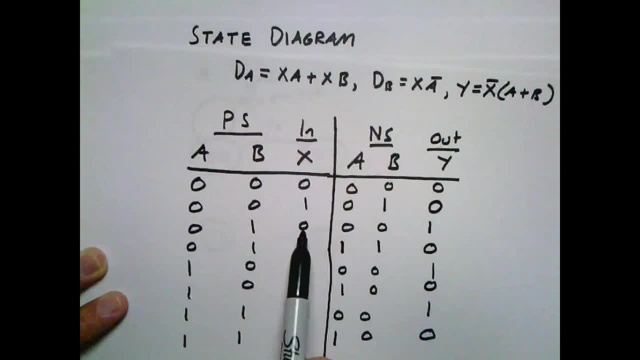 1, 0, 0, 1, 1.. If we're at 1 and we get a 0,, we go back to 0 and we output a 1.. And if we get a 1,, we go to 3. 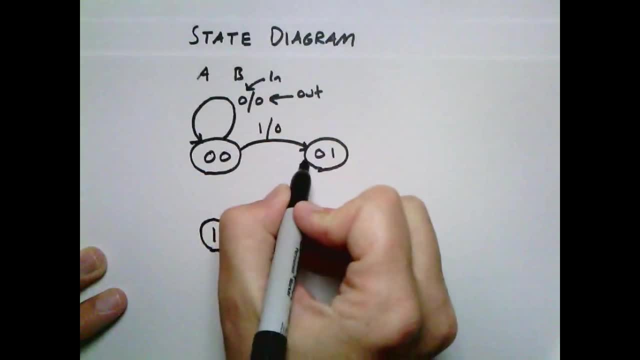 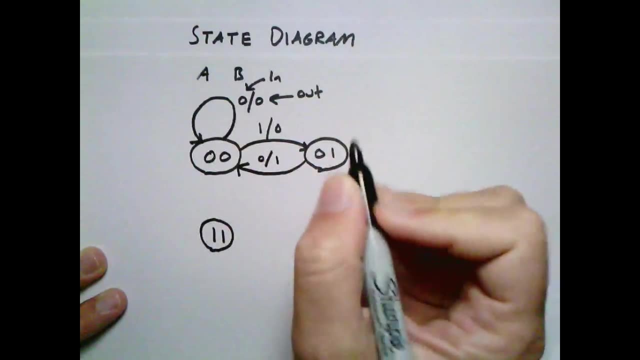 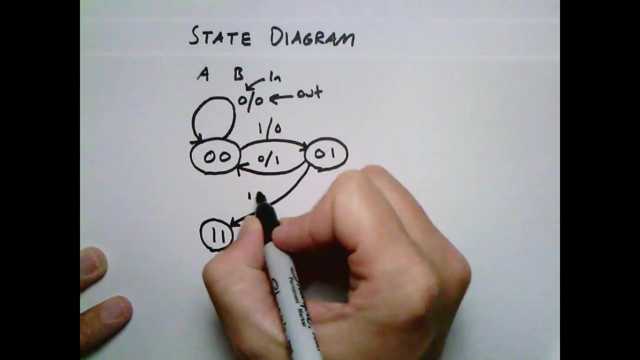 and output a 0. So we can come back to 0. That's if we got an input of 0 and we would output a 1.. Or we can go here to 3, and that's if we got a 1 and we will be outputting. 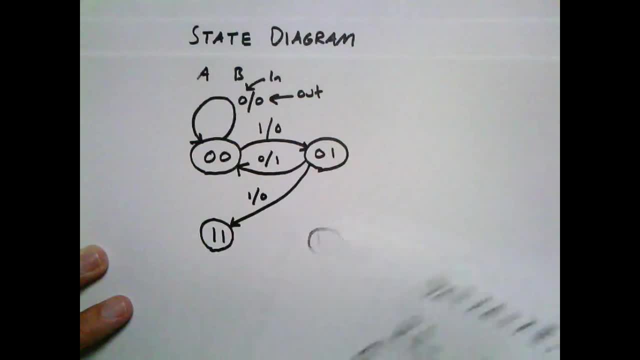 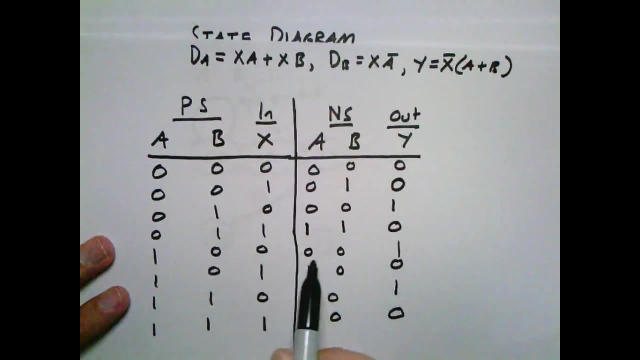 a 0.. So that's it for 0, 1.. Now let's just go down to 0, to 1, 0.. So if we get for 1, 0,, we get a 0, we go to 0 and output a 1.. 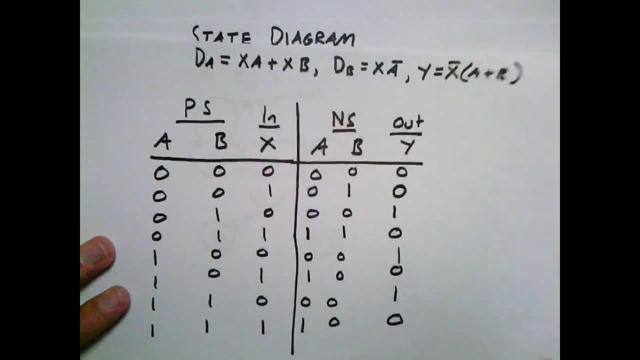 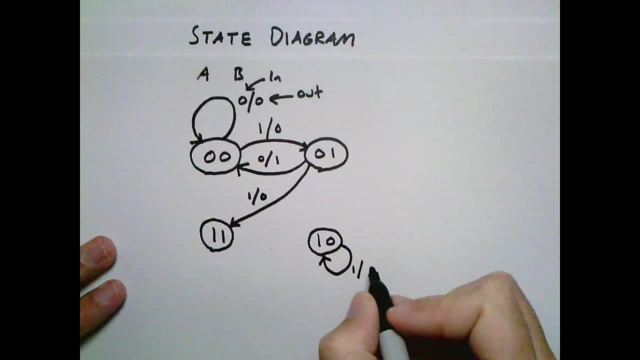 If we get a 1, we go to, we stay there and output a 0. So let's do that: If we got a 1, we would output a 0. Yeah, And if we got a 0, we would sort of. 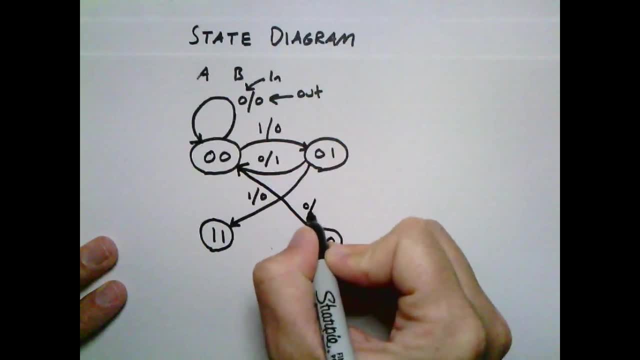 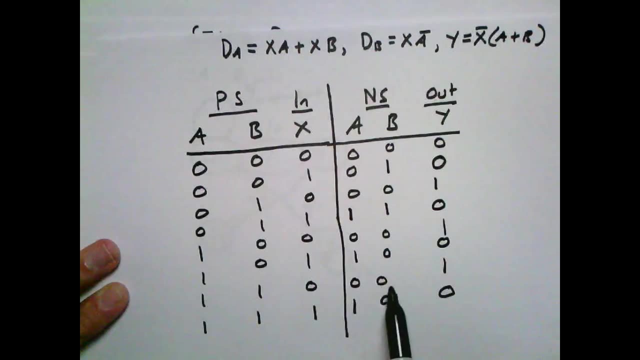 hop back in with that guy and output a 1.. And then, last but not least, at state 3, 1,, 1, if we get a 0, we go to 0 and output a 1.. If we get, 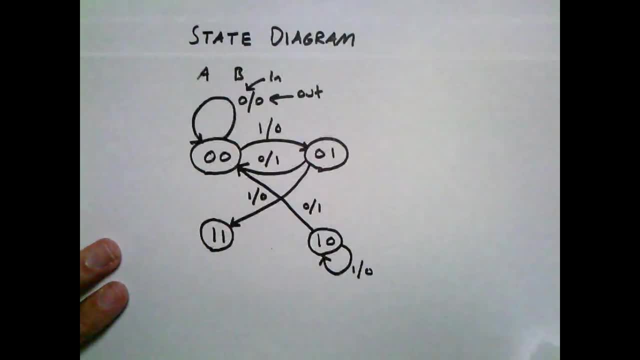 a 1,, we go to 1, 0 and output a 0. So we got that guy that was a 0, and we output a 1.. And if we got a 1, we come back to here and output a 0. 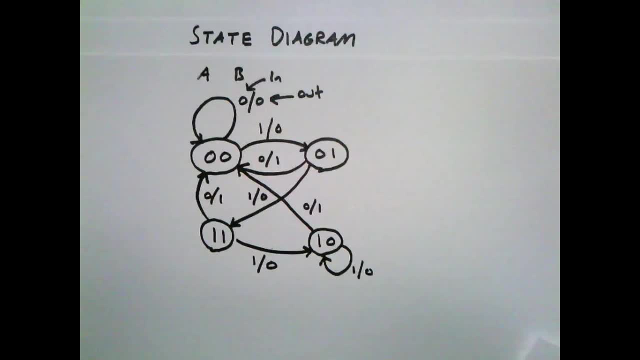 So that's 1 to 0.. So there you have it. There's our state diagram. We can see all three states and sort of a graphical representation of what happens. We get a 0, we know we're gonna stay at 0 and output a 0.. 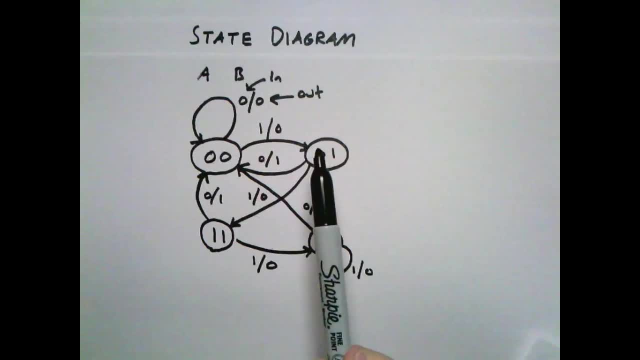 If we get a 1, we're gonna jump to state 1 and output a 0.. If we get a 0 again, then we'll output a 1 and go back to 0 and sort of start over. And you can see, you can use this. 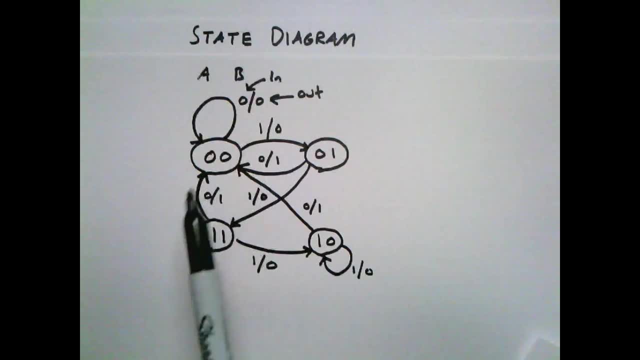 to sort of trace and sort of graphically represent and see how data and information in the context moves around inside your circuit, And that's all. there is, too. There's a couple different types of state diagrams. There's a few different types of notations.